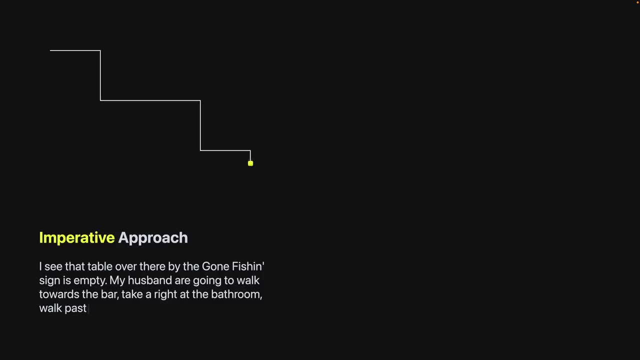 husband and I are going to walk over to the bar, take a ride to the bathroom, walk past the two tables and then walk up to the table and say: I see that table over there by the Gone Fishin' sign is empty. my husband and I are going to walk over to the bar, take a ride to the bathroom, walk past. 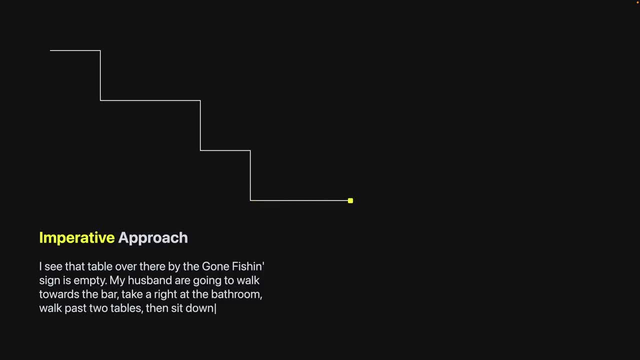 the two tables and then sit down. Another may simply look like this: You walk up to the waiter and say table for two, please. One of these approaches- the imperative approach- is focused on how you're going to get a table. The other, the declarative approach- is focused on what you want. 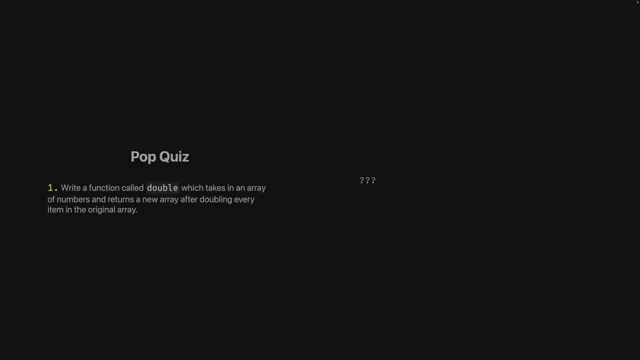 a table for two. Let's look at some code. Say we wanted to write a function called double which takes in an array of numbers and returns a new array after doubling every item in the original array. One approach may look like this, where we times each number in the original array being 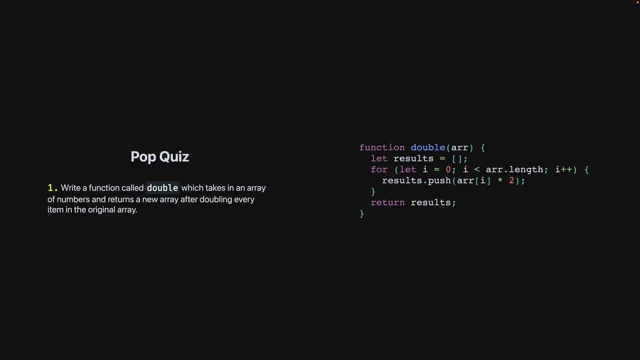 passed in by two. or we times each number in the original array being passed in by two, or we push that into the new array and then return the results. Next, what if we wanted to write a function called add which takes in an array and returns the results of adding up every item in? 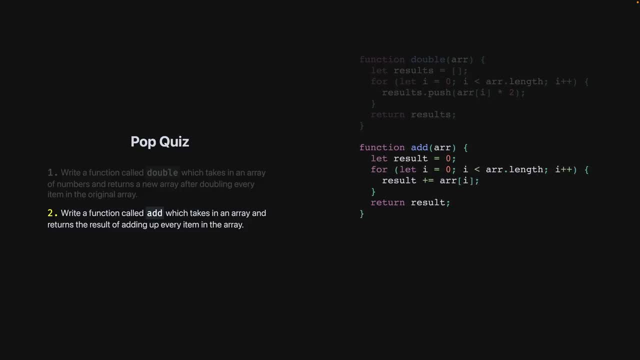 that array Again. a similar approach may look like this: where we create a variable and set it equal to zero, then we add the value of each item in that original array that's being passed in to this variable and return it Last. 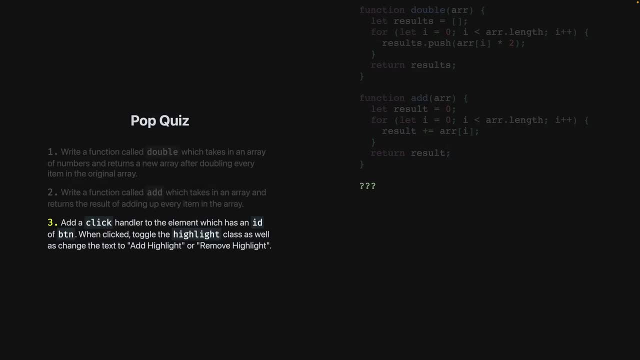 let's say we wanted to add a click handler to the element which has an id of button. When clicked, toggle the highlight class as well as change the text to add, highlight or remove highlight. One approach may look like this, where first we'd get the element that has an id of button. 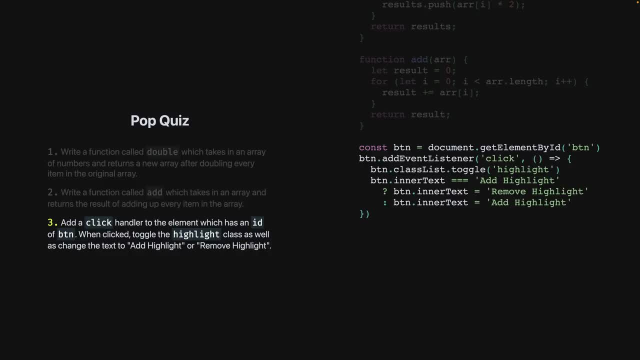 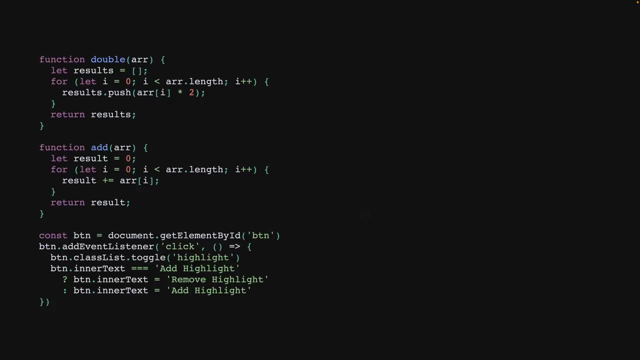 From there, whenever the user clicked the element, we'd toggle the class and, based on its current state, update its text. Now, is this code bad? Well, of course not, But in each of these examples we're conforming to the operational model of the machine. 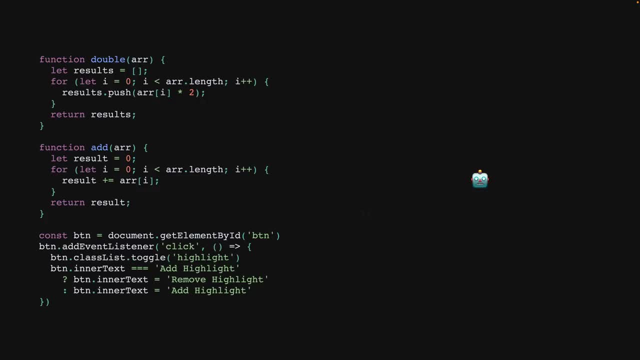 by describing how we want to accomplish a certain task, rather than what we want. Another way to think about the difference between imperative and declarative code is if you can trace the execution of the program as it runs. In each of these examples, we can very clearly trace how the program is going to run. This forces us to again: 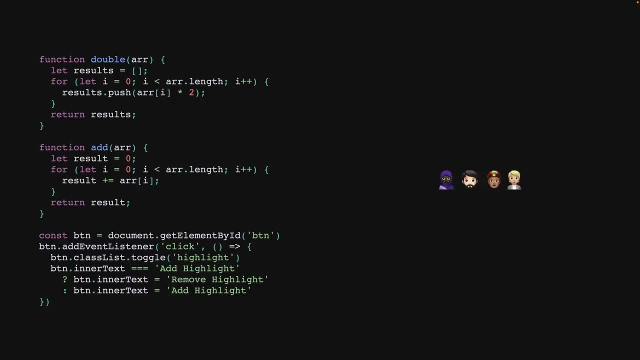 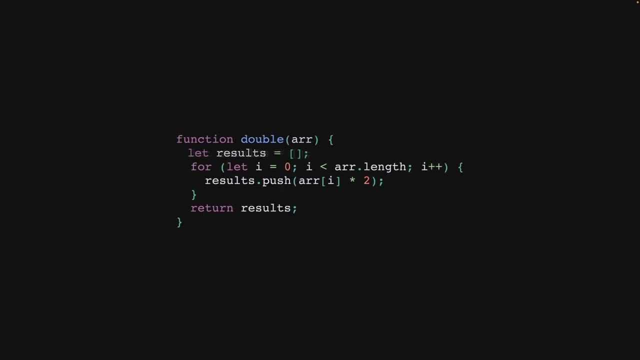 think like a computer, in a very operational way, rather than as a human. So now the question is: how can we update this code to be more declarative? Let's take a look For double. we can leverage JavaScript's map method to return a new array after multiplying.